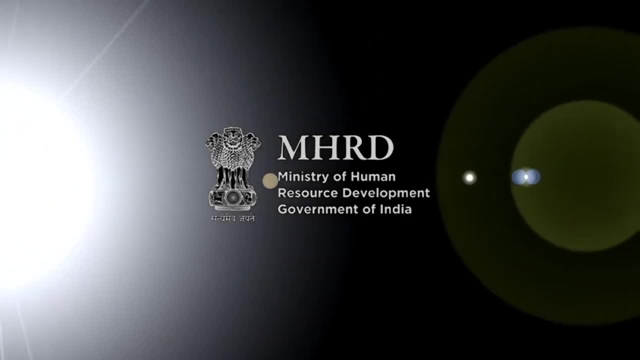 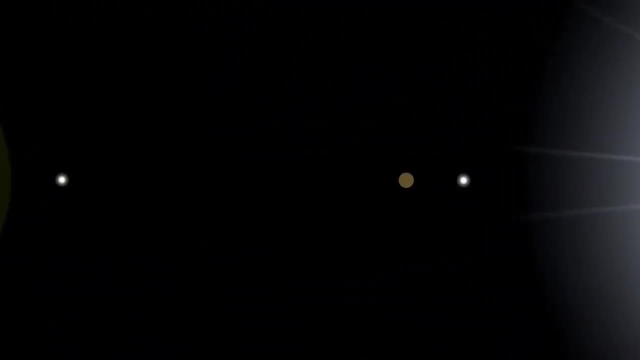 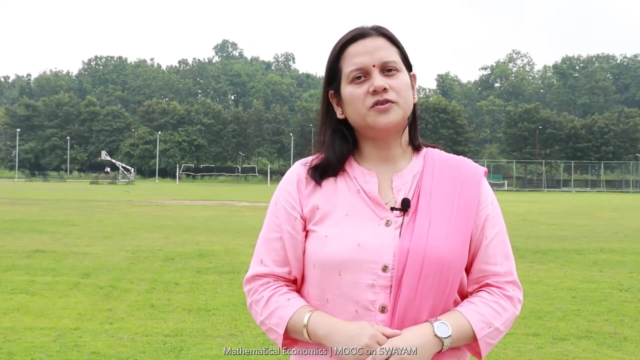 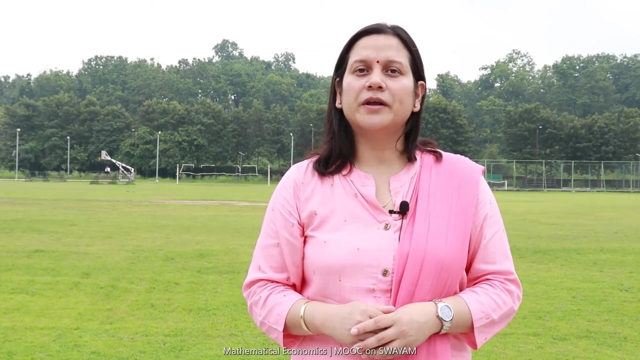 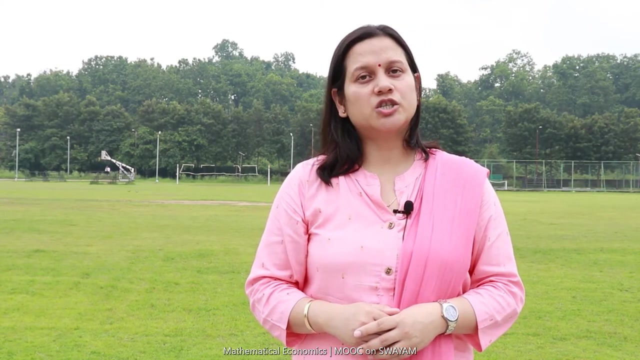 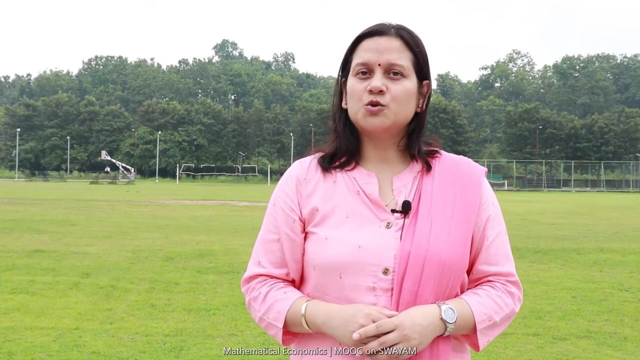 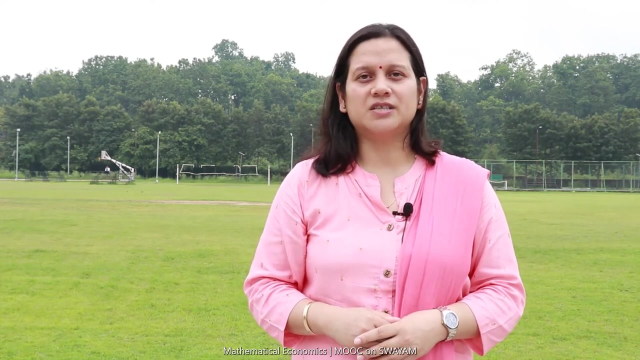 Geometry plays an important role in mathematics. Geo means earth, and metri is derived from the Greek word metron, which means measurement. Geometric interpretation of concepts such as shape, position, space, angle and curve makes complex analysis easy to understand. In this video, you will learn how to find the definite integral using geometric interpretation. 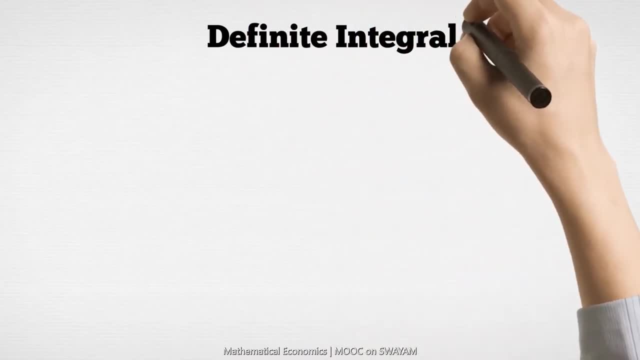 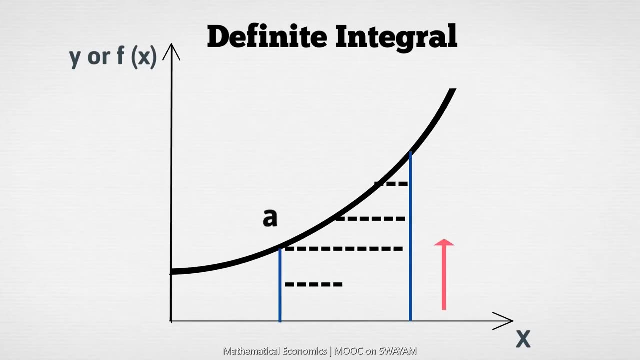 By definition definite integral represents the area under a curve, above the x axis and between two defined values: x is equal to a and x is equal to b. This is the graph of the function. y is equal to f of x and we want to find the area under this curve and above. 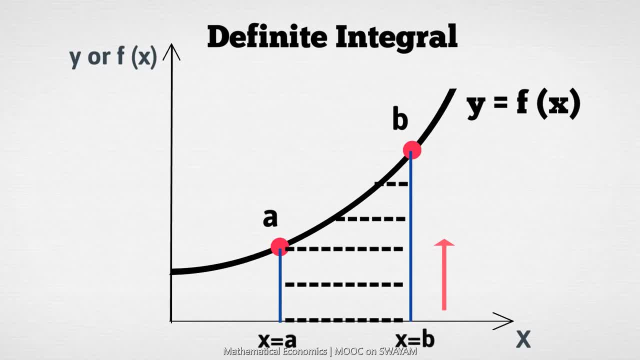 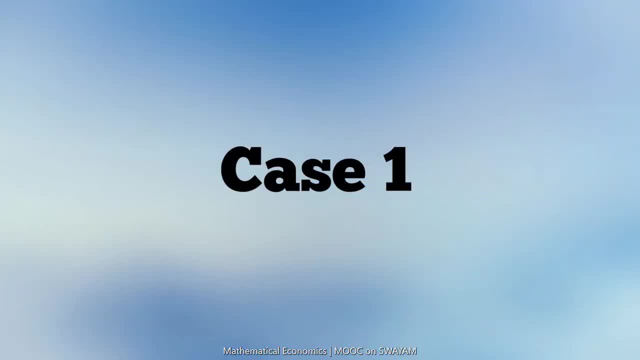 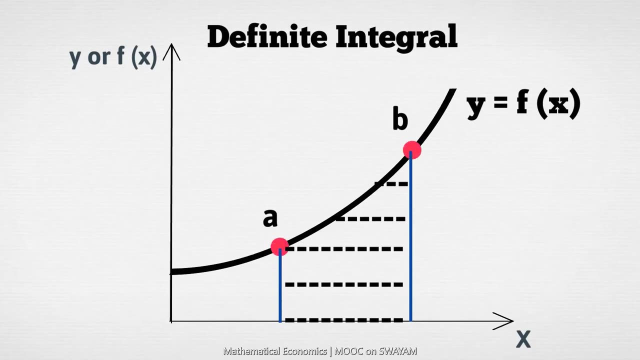 the x axis between two points, x equal to a and x is equal to b. Extending point b to meet the y axis gives the value of y. when x is equal to b, That may be represented as f of b. Then point q on this line gives the value of x. that is: 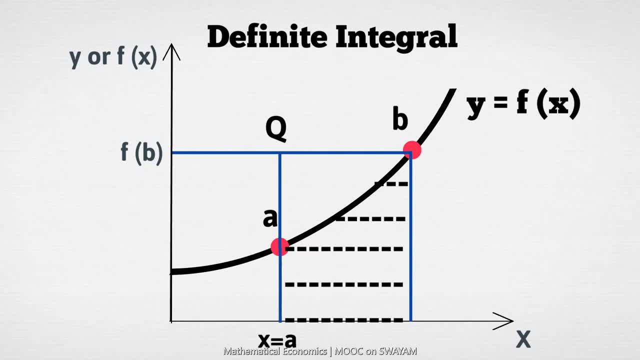 a. Now, the distance between x equal to a and x equal to b is a change in the value of x and may be represented as delta x. To find the area under the curve between a and b, we may find the area of the rectangle. 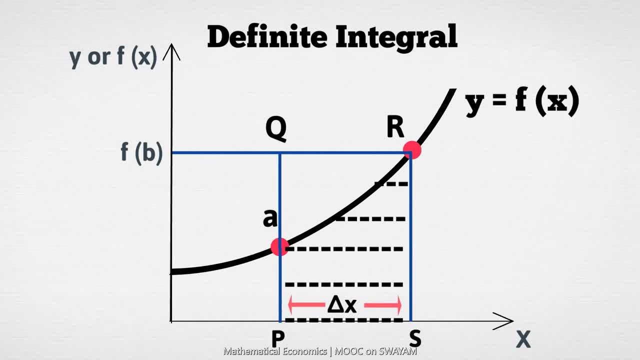 PQRS and then subtract the region AQR. With the given information can you find the area of the rectangle PQRS, Since area of a rectangle is length into breadth, and length is given by f of b and breadth is given by delta x. 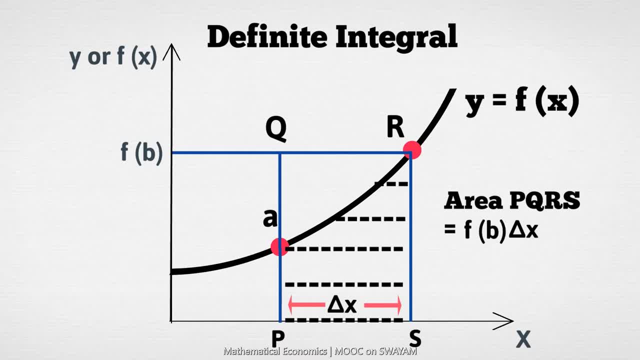 So you can see that, Similarly, the area of the rectangle is length into breadth and length is given by delta. x is greater than the area under the curve between the two points, x equal to a and x equal to b. But it is difficult to find the area of the region a, q, r because it is not a proper triangle. 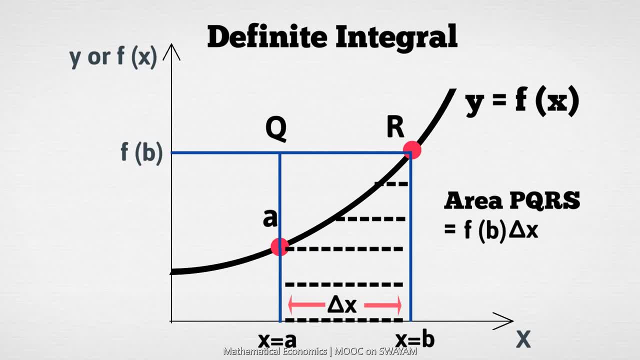 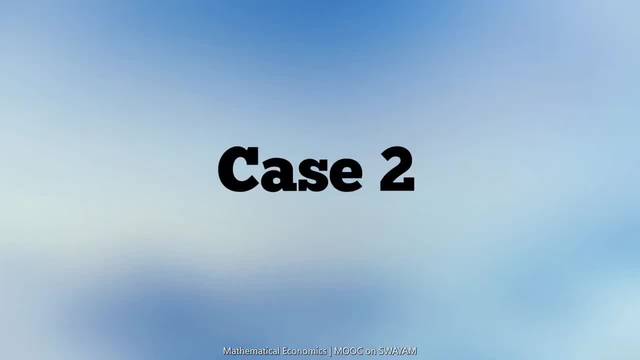 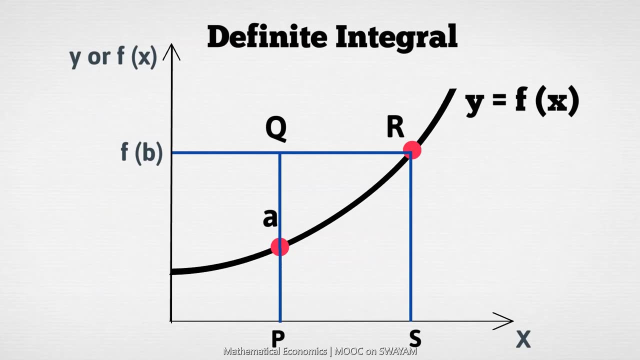 This can be solved in the second case. If we divide the rectangle p, q, r, s into two parts, we get the sum of the area of two rectangles. Let us draw a line parallel to x-axis, to the line p, w, and name it q. 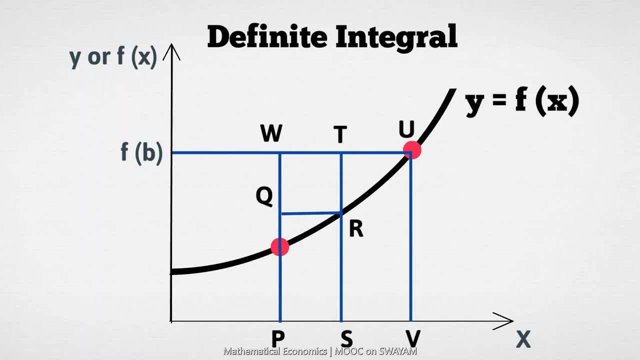 And we will get the sum of the area of two rectangles And then extend it to y-axis to get the value of y. Suppose value of y is f of a star, If the change in the value of x is delta x1 and delta x2, can you find the area of the two rectangles? 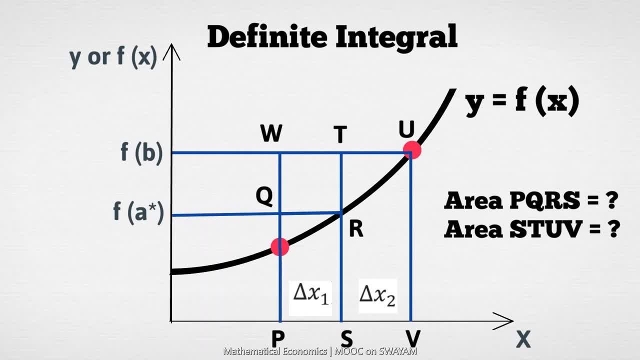 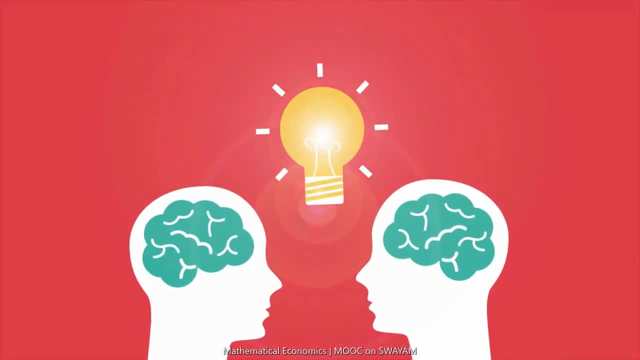 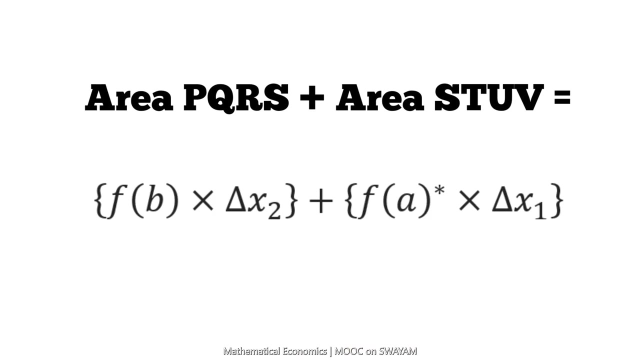 Pause the video and write the sum of the area of two rectangles. You can see the sum of the area of rectangle s, t, u, v and p q r s. This is the result You can see. the sum of the area of the two rectangles is still greater than the area under the curve. 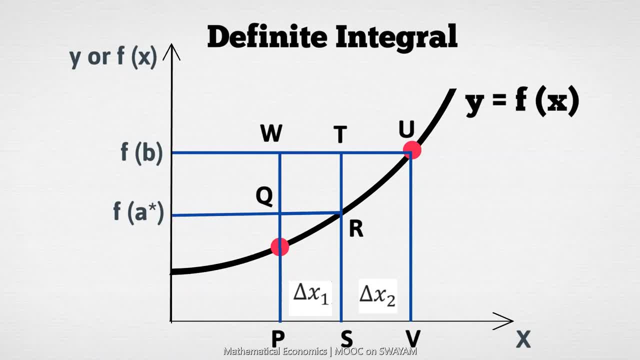 But the sum of the area of the two rectangles is still greater than the area under the curve. But there is a difference between the first case and the second case. Could you point out the difference? Yes, the region A, w, u in case 2 that was shown as A, q, r in case 1 has been reduced by the area of the region q, w, t, r. 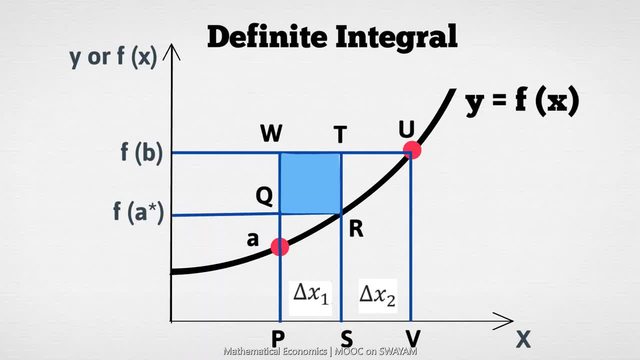 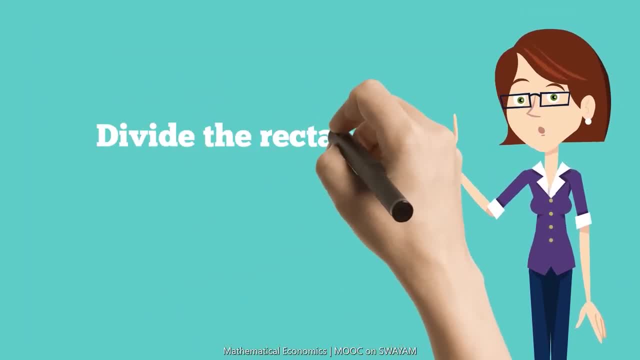 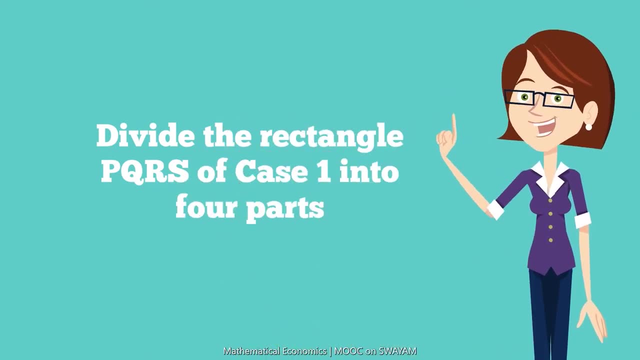 This has helped us in moving a step closer to the equation. It is the area under the curve. Now consider a third case. Divide the original rectangle P, q, r, s of case 1 into four parts. What is the result?